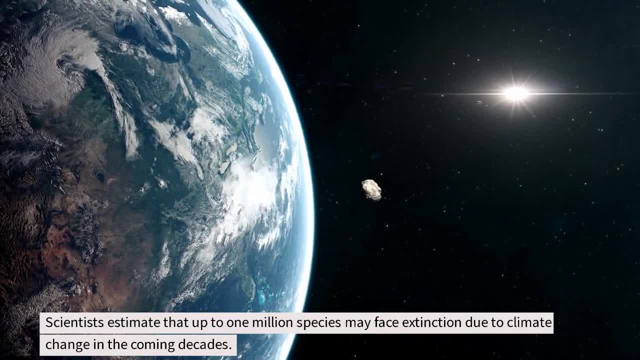 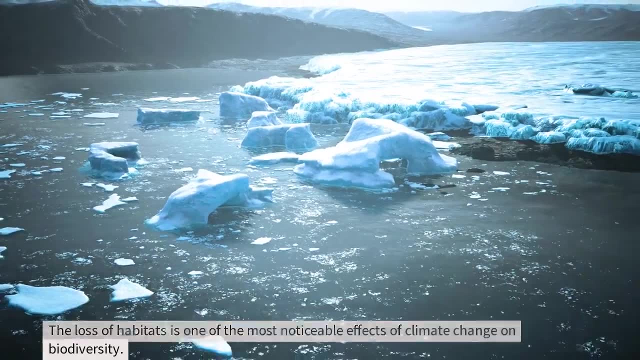 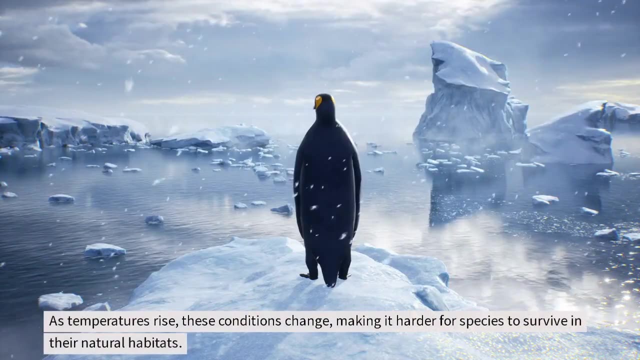 to one million species may face extinction due to climate change in the coming decades. The loss of habitats is one of the most noticeable effects of climate change on biodiversity. Many animals, plants and insects depend on specific environmental conditions to thrive. As temperatures rise, these conditions change. 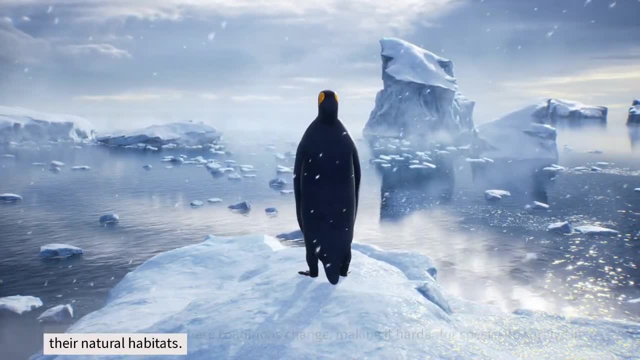 making it harder for species to survive in their natural habitats. This reduces the number of species that survive in their natural habitats. This reduces the number of species that survive in their natural habitats. This reduces the number of species that survive in their natural habitats. 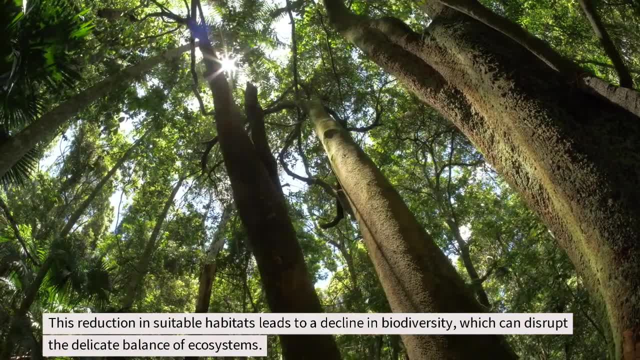 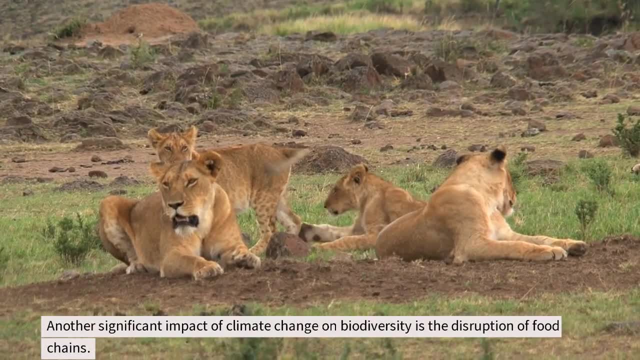 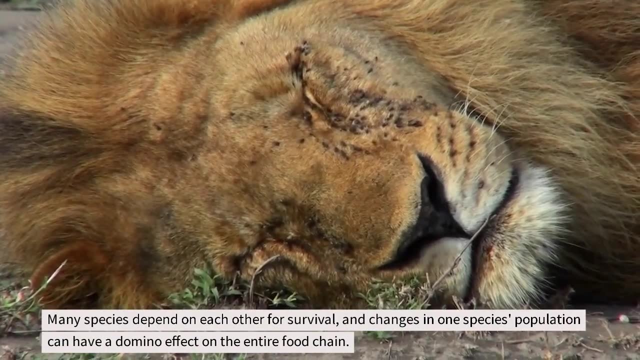 The reduction in suitable habitats leads to a decline in biodiversity, which can disrupt the delicate balance of ecosystems. Another significant impact of climate change on biodiversity is the disruption of food chains. Many species depend on each other for survival and changes in one species' population. 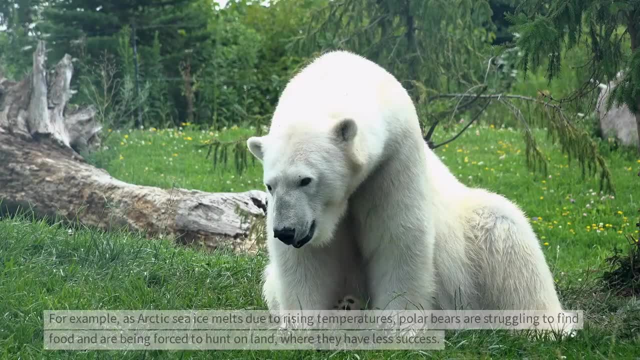 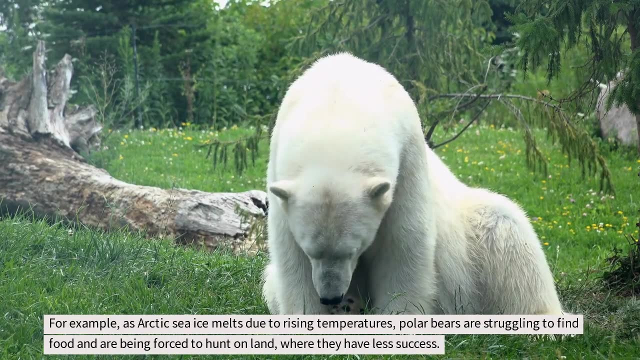 can have a domino effect on the entire food chain. For example, as Arctic sea ice melts due to rising temperatures, polar bears are struggling to find food. For example, as Arctic sea ice melts due to rising temperatures, polar bears are struggling to find food. 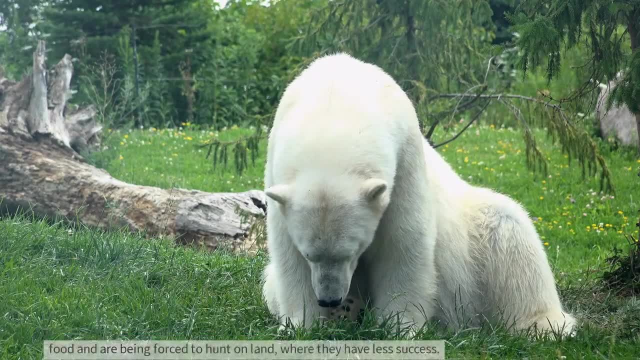 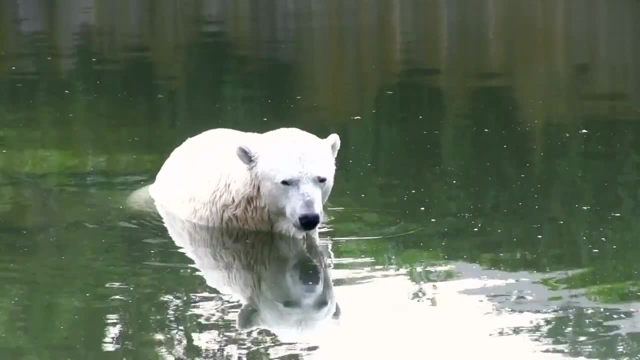 And are being forced to hunt on land where they have less success. This can lead to a decrease in the polar bear population, as well as a decline in the populations of their prey. Climate change also has a profound impact on migratory birds. Many species of birds rely on seasonal patterns for breeding, migration and food sources. As temperatures change, these patterns can be disrupted, leading to a decrease in the number of birds that breed or migrate to certain areas. This can also lead to an increase in competition for resources. 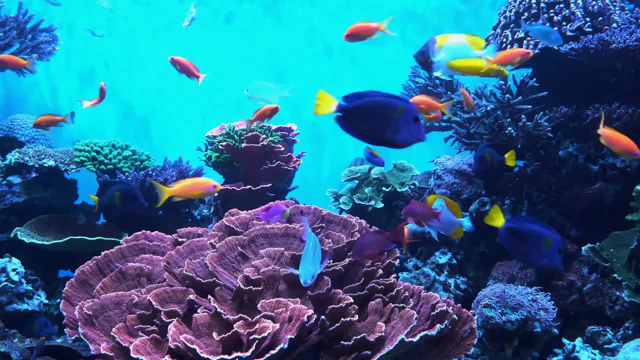 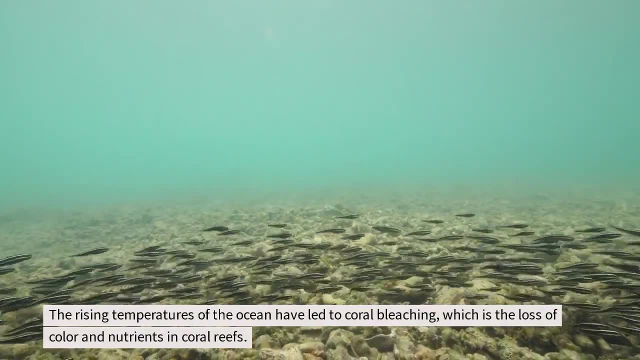 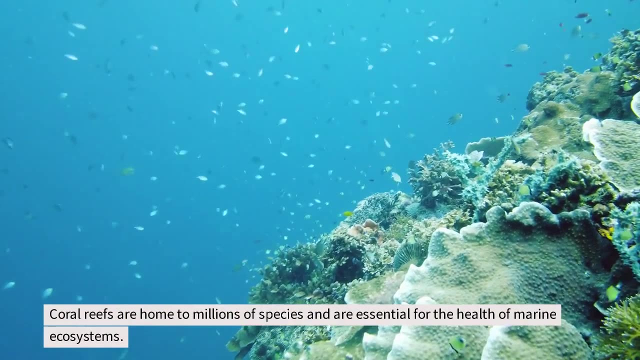 which can have a negative impact on bird populations. Furthermore, climate change affects marine ecosystems. The rising temperatures of the ocean have led to coral bleaching, which is the loss of color and nutrients in coral reefs. Coral reefs are home to millions of species and are essential for the health of marine ecosystems. 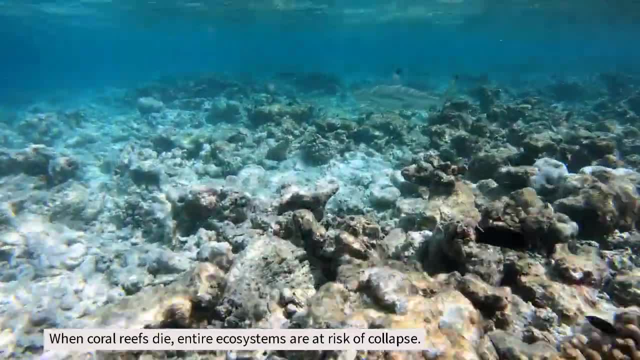 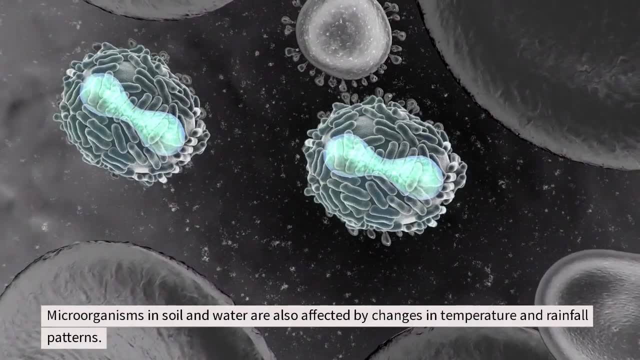 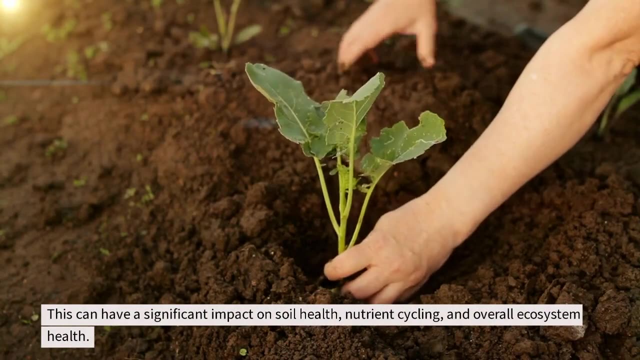 When coral reefs die, entire ecosystems are at risk of collapse. It's not just animals and plants that are impacted by climate change. Microorganisms in soil and water are also affected by changes in temperature and rainfall patterns. This can have a significant impact on soil health, nutrient cycling and overall ecosystem health. 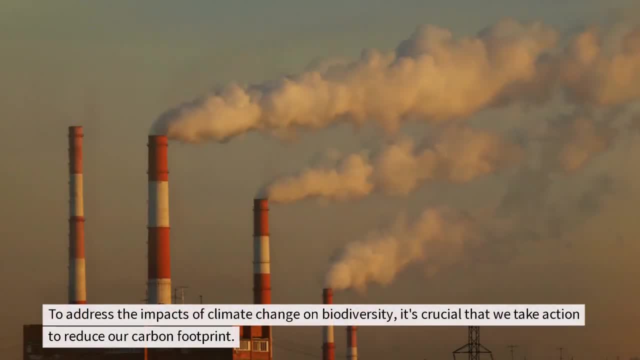 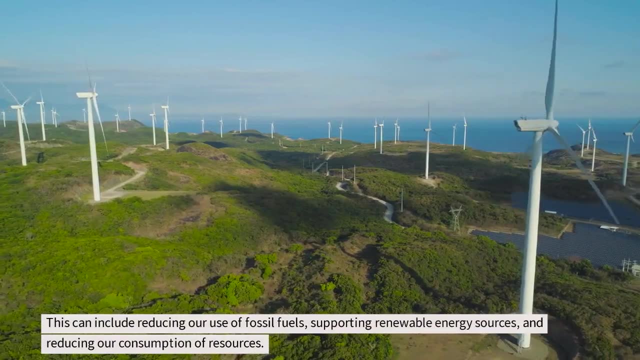 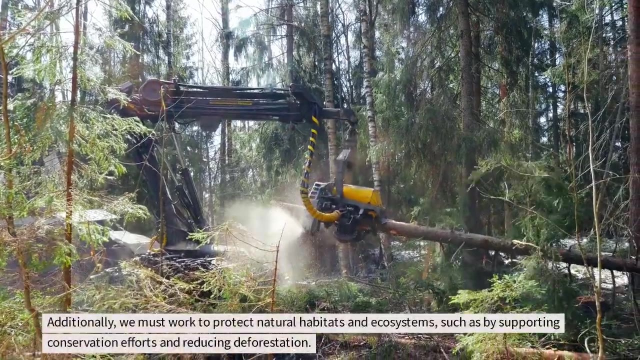 To address the impacts of climate change on biodiversity, it's crucial that we take action to reduce our carbon footprint. This can include reducing our use of fossil fuels, supporting renewable energy energy sources and reducing our consumption of resources. Additionally, we must work to protect natural habitats and ecosystems.